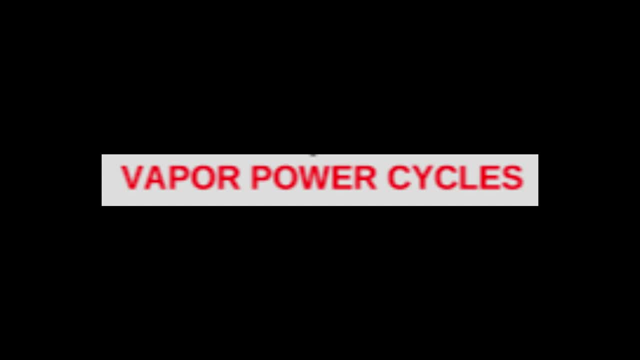 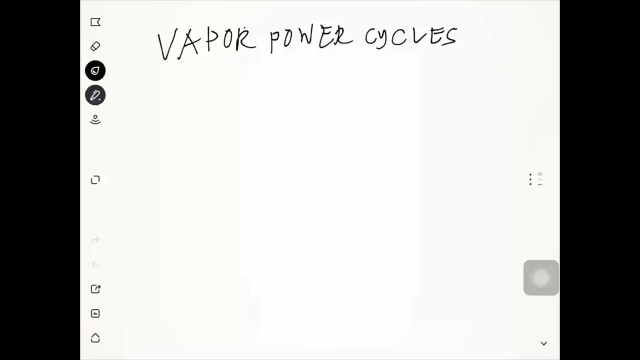 are commonly referred to as coal plants, nuclear plants and natural gas plants. Steam is a type of fuel used to supply heat to the steam. However, the steam goes through the same basic cycle in all of them. Therefore, all can be analyzed in the same manner. 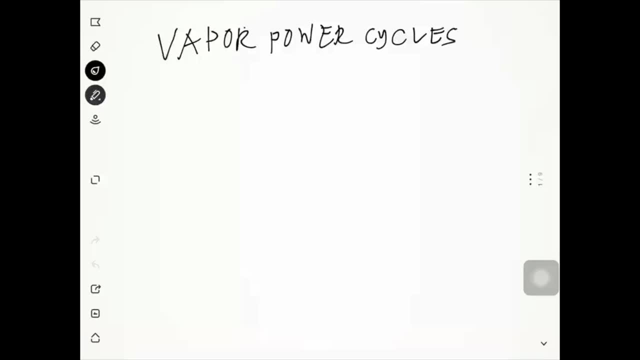 So we will discuss the highest performance or the highest efficiency of steam. The highest efficiency of steam is the current vapor cycle. Given the two operating temperatures, we have the two reservoirs. Given the high temperature. for example, this is our heat engine. 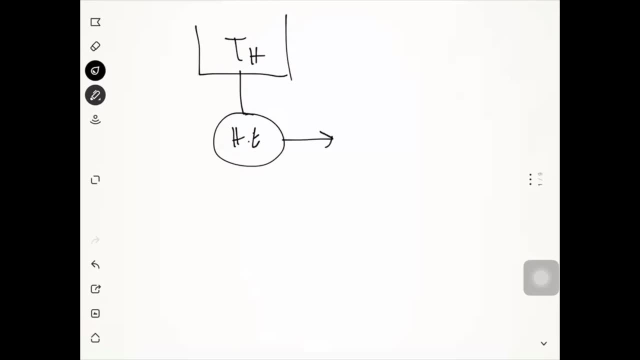 it will generate work, And this one, this is our T-L. So this is our Q-H and our Q-L. So we discussed or we derived the thermal efficiency, which is the work efficiency, Work net over the Q-N or the Q-H. So, in terms of temperature, our thermal efficiency will 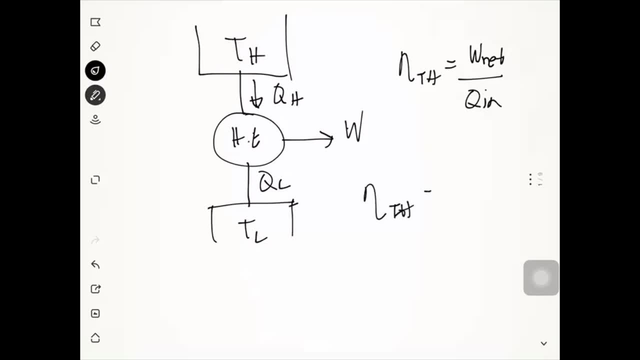 be. this is 1 minus T-L over T-H, So this efficiency has the highest is the highest so far, based on the second law. in a machine that has the highest efficiency, Then the kernel cycle is a violation of the second law of thermodynamics. 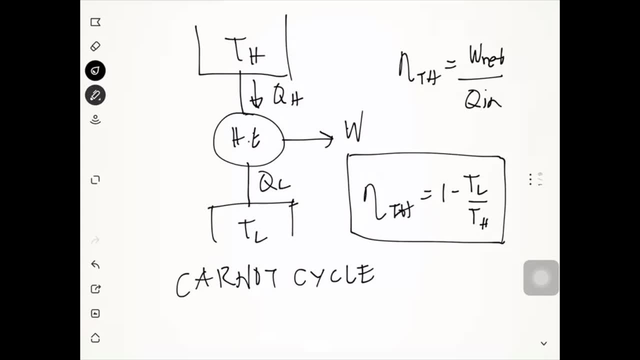 So we will evaluate the kernel cycle if it is really applicable for the vapor-power cycle. So first we will evaluate the vapor-power cycle Draw, we will draw the T-S diagram, The T-S diagram for our kernel cycle, that one Okay. 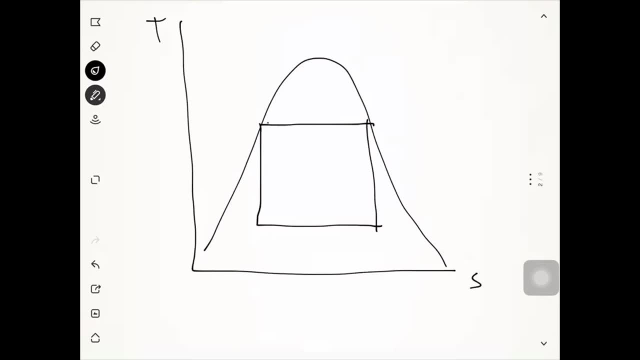 So this is our point, Okay. Okay, This is our point one and this is our point two here. point three and point four: Okay, The process one and two. This is isentropic. This process one and two is isentropic and process two to three is isothermal. 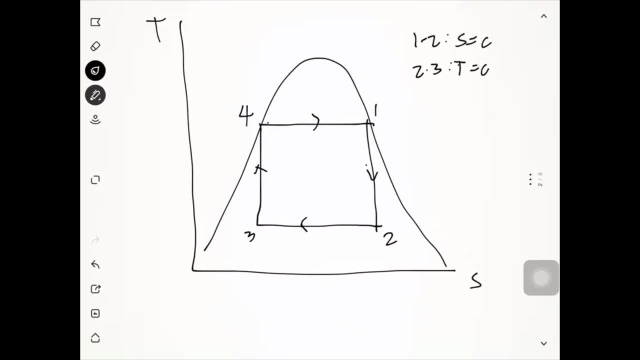 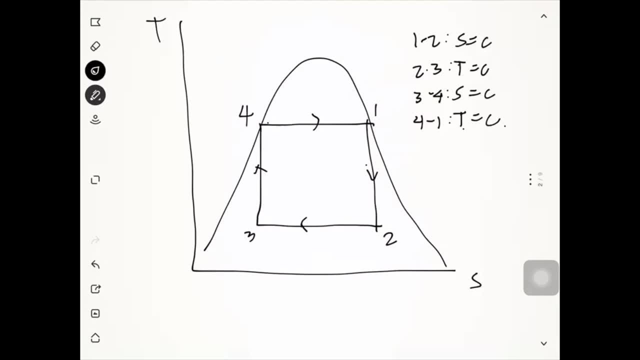 which is very complicated. Okay, critical point. okay so, but the process 1 to 2, which is isentropic- isentropic, we assume that is an isentropic for our Carnot cycle. this is the diagram for the Carnot cycle. okay, so this thing expands here from 1 to 2, then the most there is. 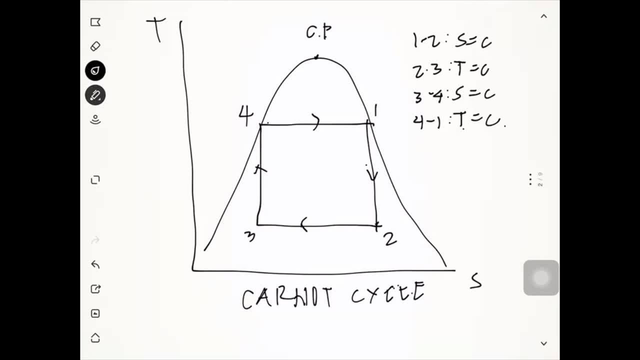 the quality of at point 2 is lesser than, or it has. the moisture content at point 2 is of, it has a higher value. so for a turbine, the causes for erosion, the causes of erosion for the turbine blades can contribute to damage. that's only a limit. it has a limit of 90% quality. 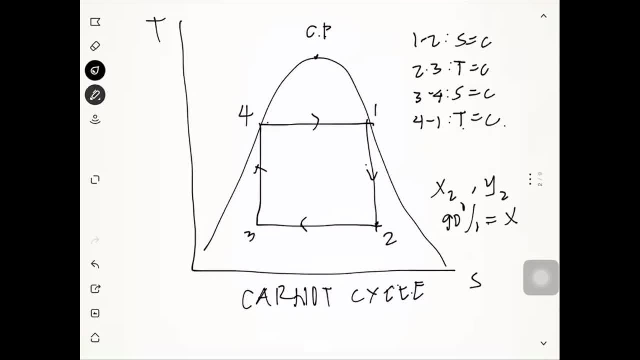 90% quality or 10% moisture content. beyond greater than 10% moisture furniture, you can damage the turbine blades. so it cannot be. it's impossible for this process from 1 to 2 to be applied in the vapor power cycle. another thing, uh, the process 2 to 3. 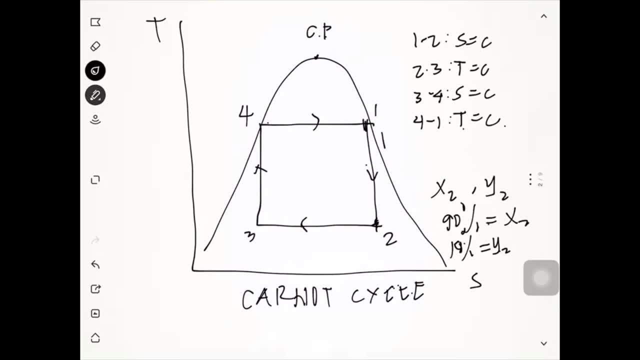 this is isothermal, So we need to have controlled quality here. at 0.3. We are going to raise its pressure to the boiling pressure from here, And this is a mixture of liquid and vapor. So there's no device nowadays that can handle two phase, which is the liquid and vapor phase. 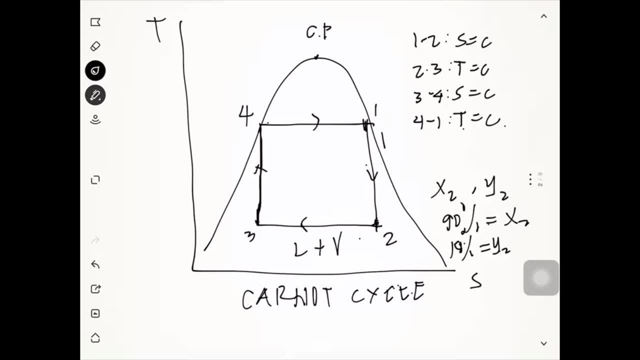 Like, for example, the pump. We know that pump handles only liquids. So if we will allow or we are going to use the kernel cycle, So we are to purchase a special pump that can handle liquid and vapor, And we have no special pump right now in the market. 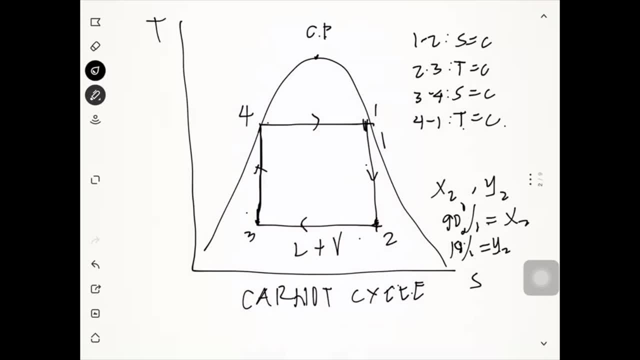 So, in short, the kernel cycle is impossible. It cannot be used in the vapor or power cycle. Okay, So what we can do now is since, for example for this one, This is the saturated liquid line and the vapor line here. So since liquid, it's pump, So that one. 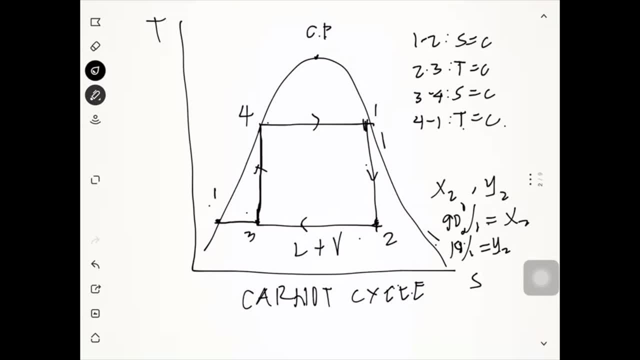 And we're going to raise its pressure, The boiling pressure, And here to improve the quality of our steam. That one. Okay, As you can see, this is our 3 prime and this is our 2 prime. So in this diagram we have inserted the 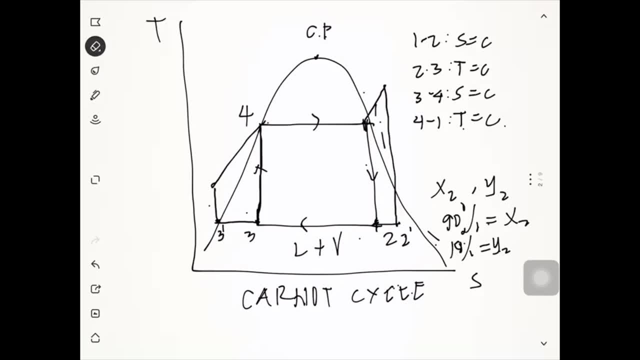 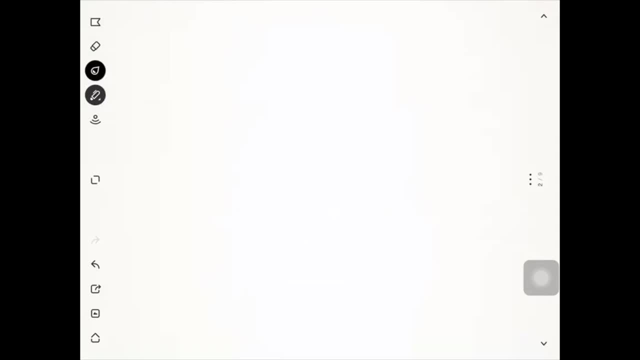 at 0.3 prime. it's pure liquid. Okay, So, as we're going to draw, it's the diagram for this one, This diagram, Okay So, Okay, I'm going to draw the diagram for this one, This one. 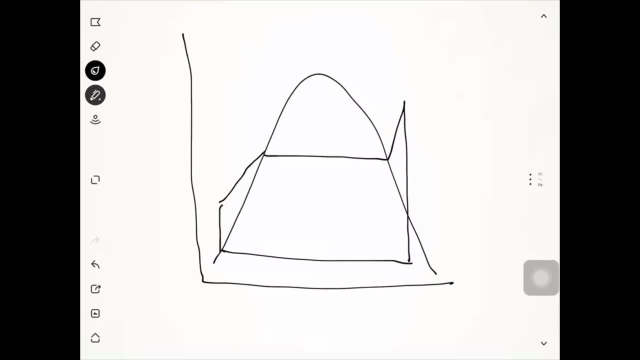 This is our 0.1,, 0.2,, 0.3, and 0.4.. This is our TS diagram. So this diagram, here is what you call. This diagram, here is what you call. This diagram, here is what you call. 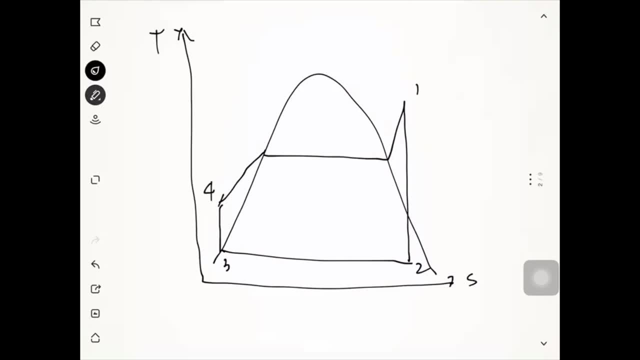 Our Rankine cycle. So for vapor power cycles Rankine cycle has the highest efficiency. So it is still ideal. because we assume here ideal processes, Like for example, process 1 and 2 is isentropic and this is 2 to 3 is isothermal, we have equal temperature. 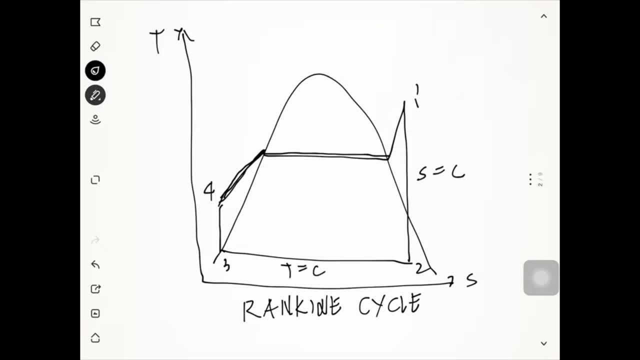 and process 3 to 4 is also isentropic. So we have now the diagram, that is diagram, the analysis for the Rankine cycle. So here is the, the ideal cycle for the proper cycles in the Rankine cycle. So these are the components. 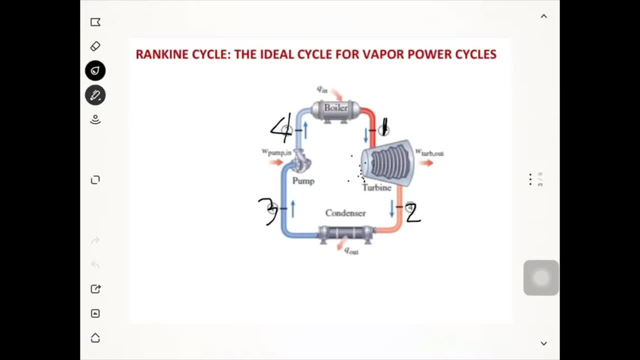 we have a boiler, we have a turbine, we have a condenser and a pump. This is a loop. We have a mass here, mass of our steam. So we have a mass here, mass of our steam. So we have a mass here, mass of our steam. 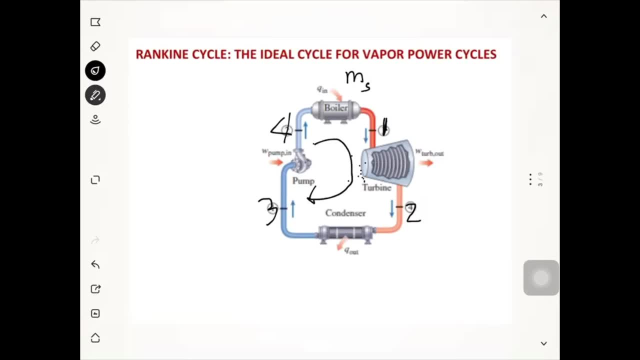 And we have the QN in our boiler and we have the work output in our turbine and we have the work input of our pump right here. So to solve the efficiency for the thermal efficiency for the Rankine, this is the same as simple: the WorkNet over the QN in 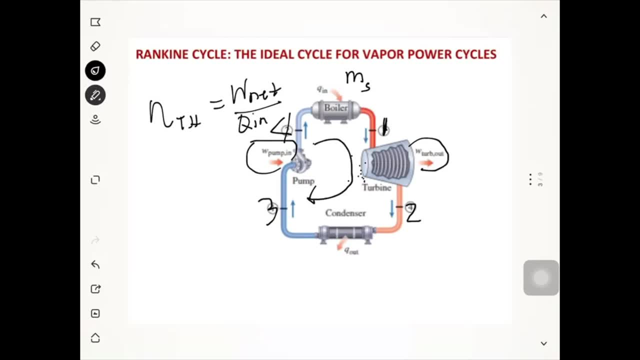 Where in our WorkNet, here is the work over turbine minus the work over pump, you have work input of our pump. So this is the work input of our pump. So we add the Q in our Map and we will donc recognizing that over the Time we have the 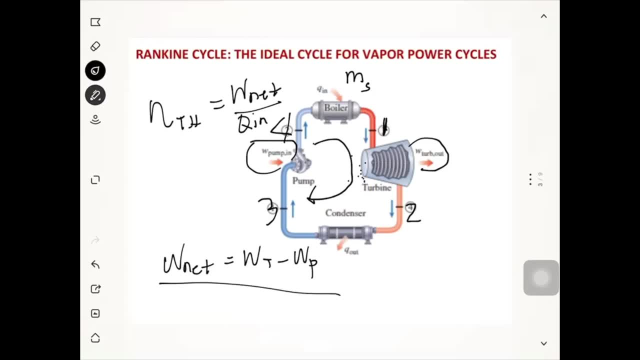 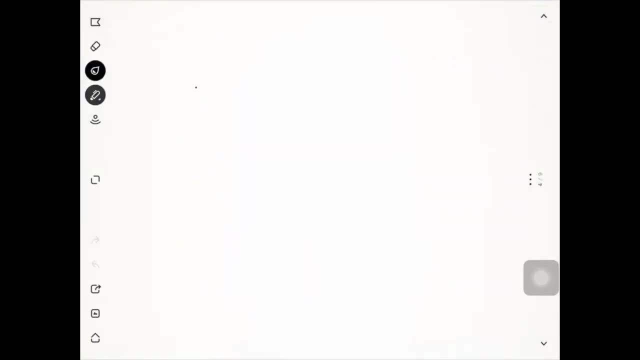 work in taking the work in and from now we are just plug anduster, so we are just falling that one, okay, okay. so in terms of enthalpy, we have the efficiency, the thermal efficiency of our rankine. we have this work net over the q n, or here it is. 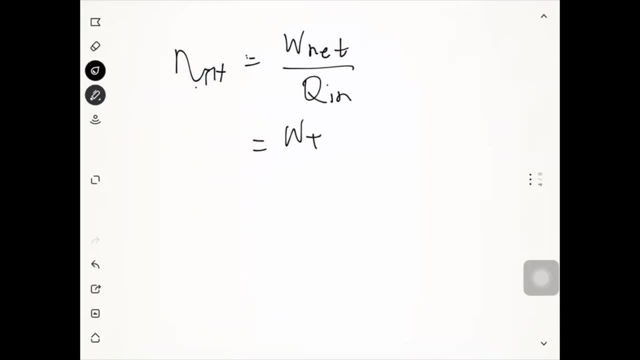 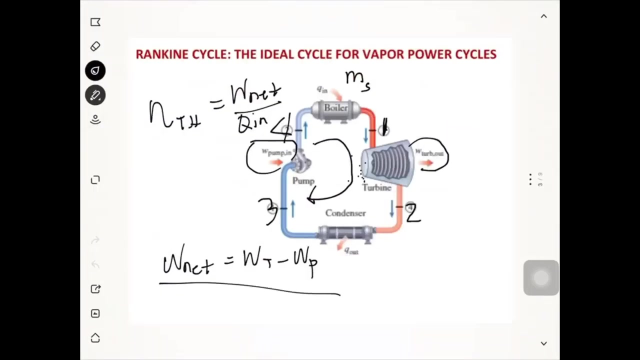 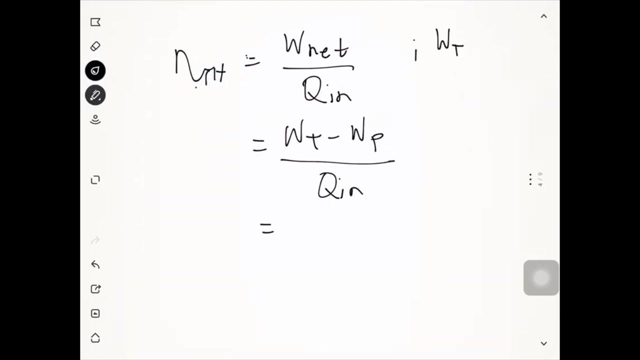 work over turbine, minus the work over pump, over the q in, or this is we have that enthalpy. in terms of enthalpy, we'll solve that one i will drive in terms of enthalpy. so we're in. our work over turbine will be. 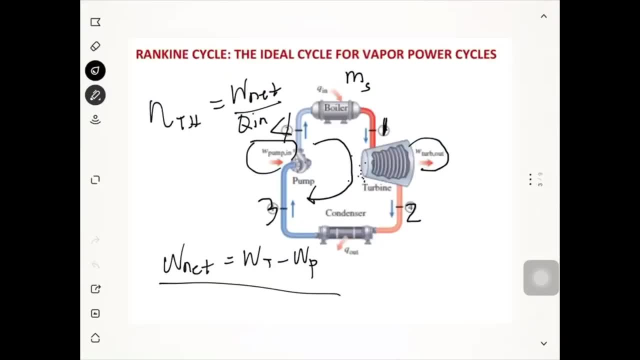 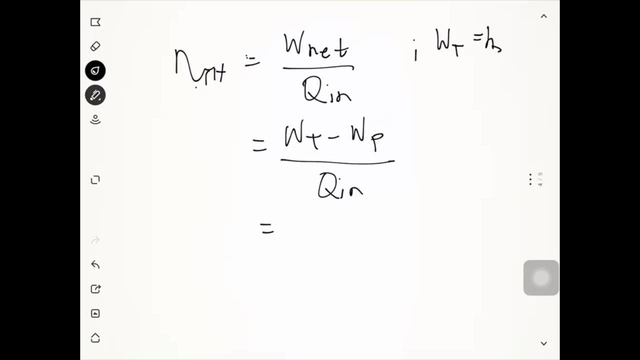 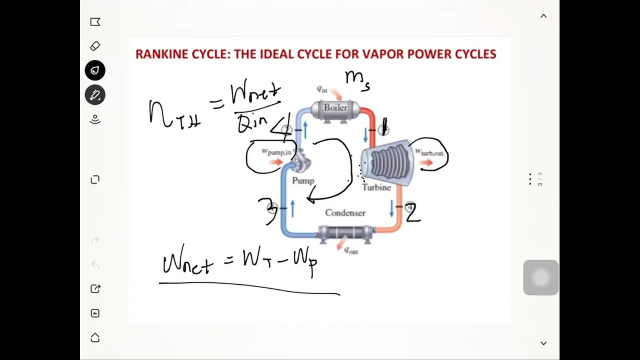 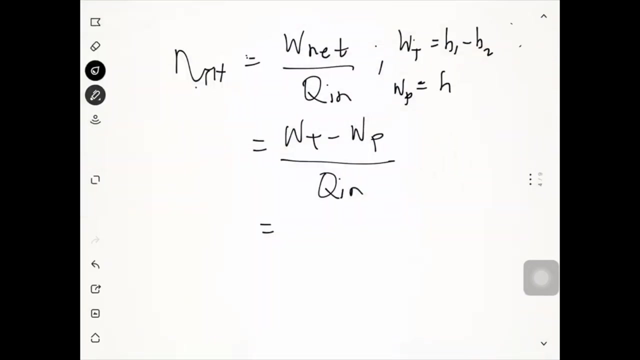 this one, that is h1 minus h2- h1 minus h2, where our entropy is in per kilogram and our wp or the workable pump, will be um. this one- this is the workable pump- will be h and it's h, that is h. 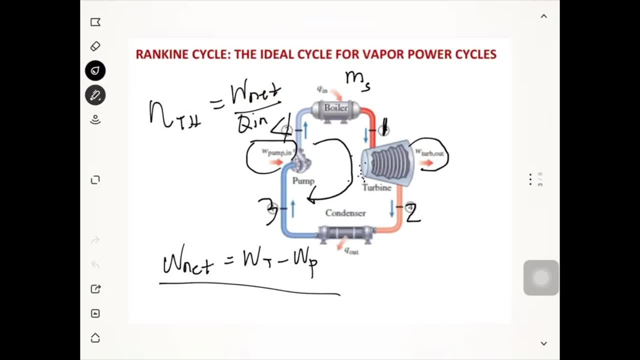 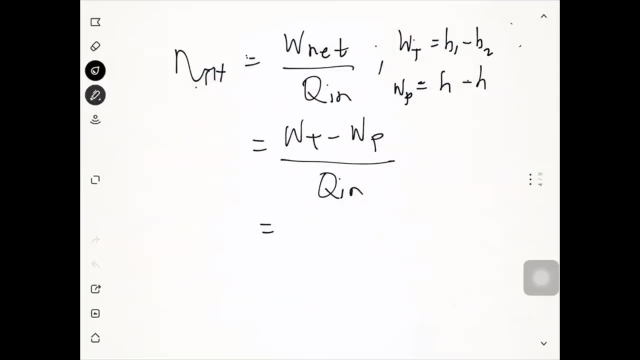 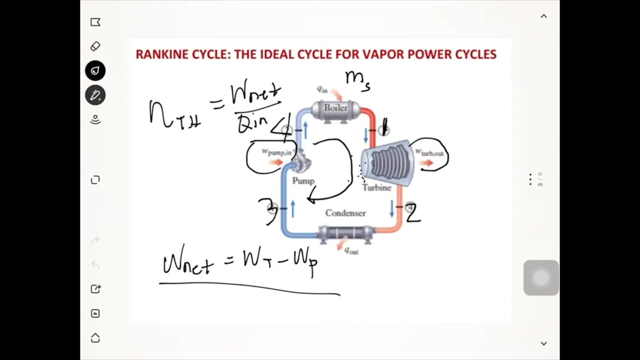 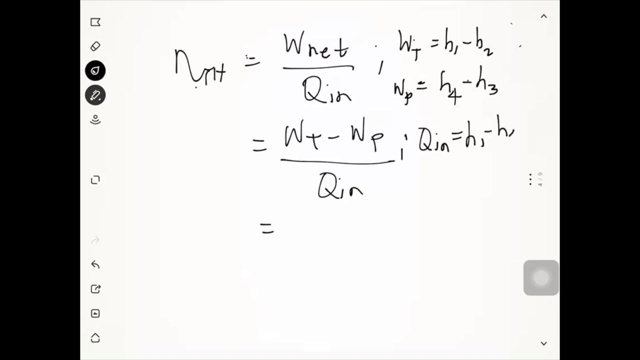 it's the work over pump. that is h3. okay, it is h4 minus h3 and our qn would be. qn would be this one: we have the h1 minus h4. so these equations, we assume that it is in the steady state, steady flow process. 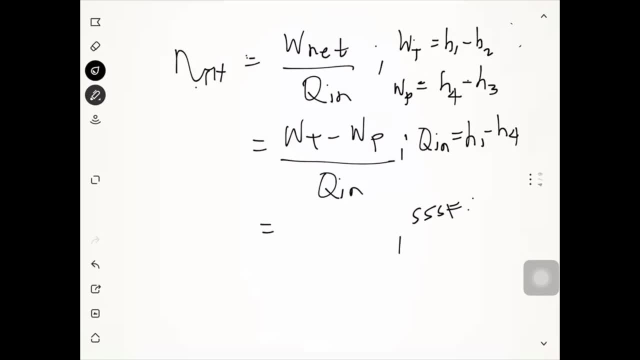 and we have the. uh, i assume that the energy in is equivalent to the energy out. okay, so our thermal efficiency would be in terms of the enthalpy, which is h1, h1 minus h2, minus the work over pump, which is h4 minus h3. 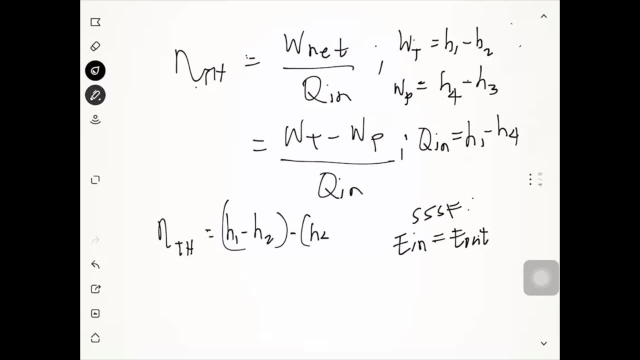 over the work in heading 2 and h1 minus h2. work in this is H1 minus H4,. okay, So we have also another equation for the pump. So in our discussion, in our previous discussion, we have workable pump would be VF3, this is: 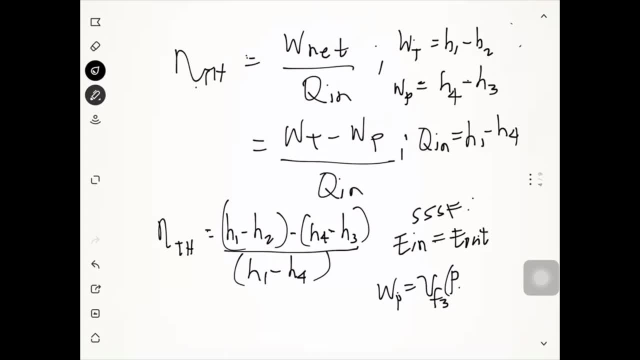 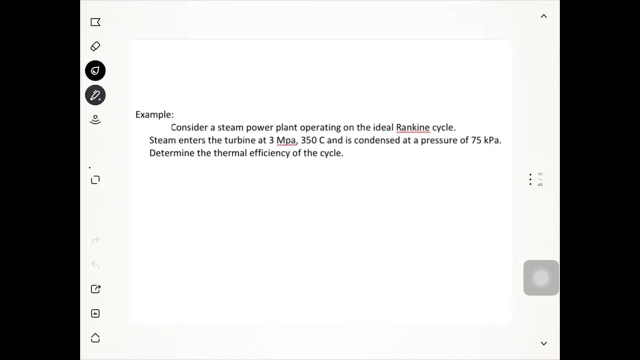 pressure at 0.4, minus pressure at 0.3, okay, So. So let's have now an example. okay, So consider a steam power plant operating in the ideal Rankine cycle. Steam enters the turbine at 3 megapascal, 350 degree Celsius, and is condensed. 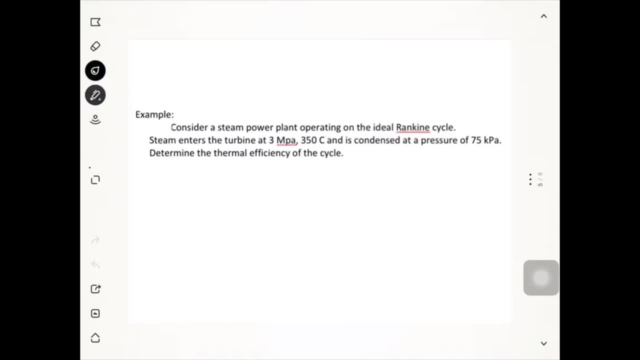 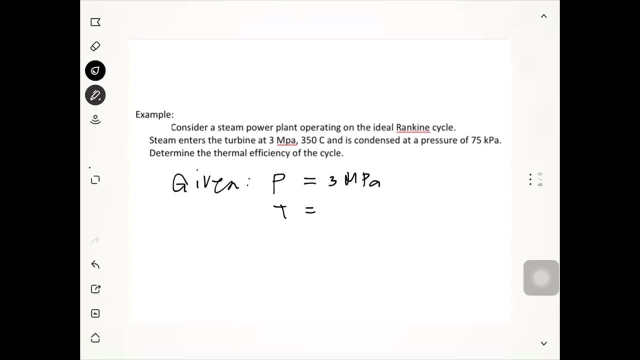 the temperature of 350 degrees celsius and we have the pressure of the condenser, which is the pressure p1. p1 pressure of the condenser is 75. we have this p2 of 75 kilopascal. okay, so we're going to draw it's. 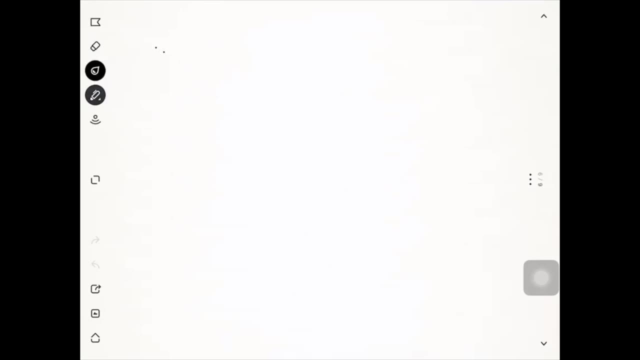 the schematic diagram. this is our boiler here and that's our turbine and this is our pump and this is our condenser and this is our pump and this is our condenser turbin, this condenser and this is our pump. you have work inputable pump. 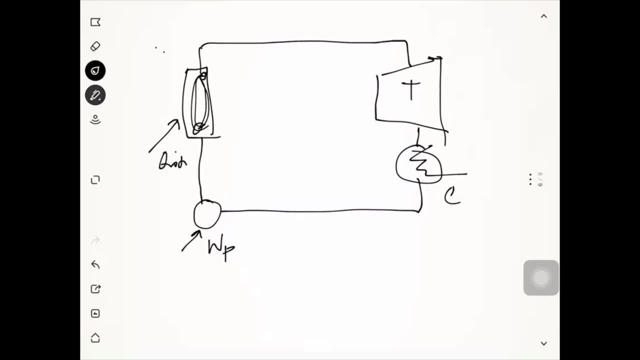 and we have the qn and turbine will generate its work. so we have this is a loop, then we have the mass of it and then we have the mass of having a body of it, steam. okay, so, based on the given from steam tables here, find the values from: 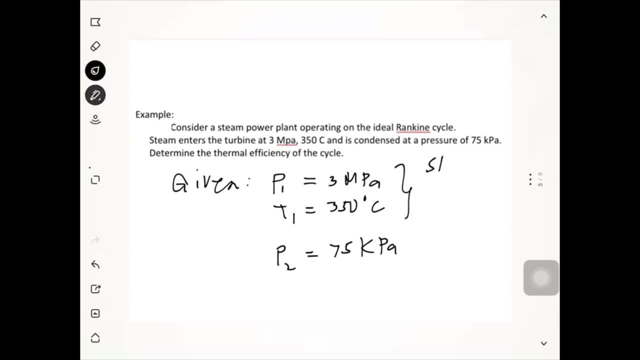 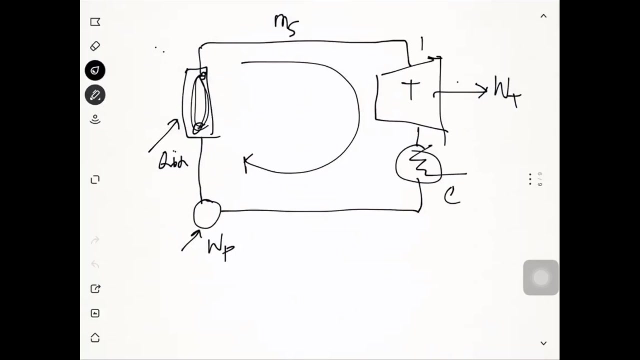 steam tables, or the mullier chart, or the intel pay versus entropy chart, the hs chart, okay, so this is our point one, two here, three and four. okay, and let's draw its th diagram for analysis. so this is the ts diagram for our rank and cycle and we assume 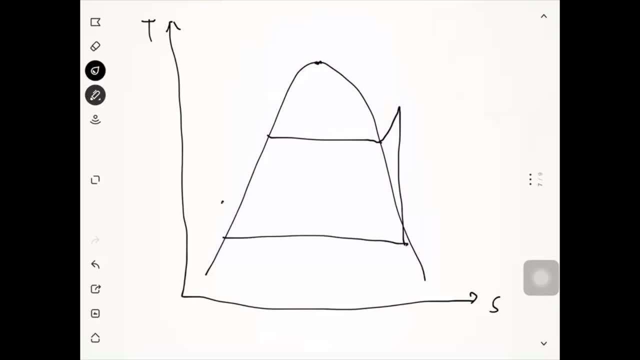 processes to be ideal. okay, point one, point two, point three at this point and point four at that point. okay, so we need to find the values for h1, values for h2, h3 and h4. so h1 is the enthalpy at three megapascal. 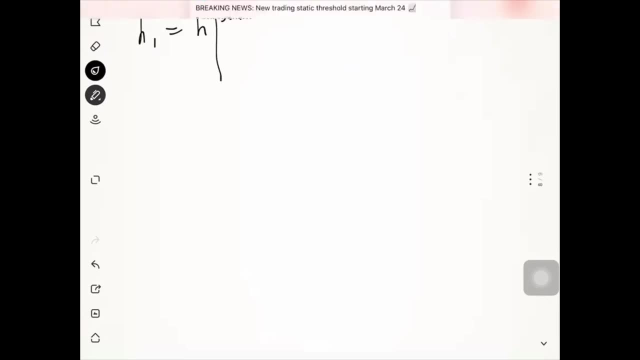 and 350 degrees celsius and we have h1 from steam tables. that is, let this superheated, non-superheated tables, we'll find the value. the value would be seven, right, two, three, two, three. Let's try to look the value for that one. 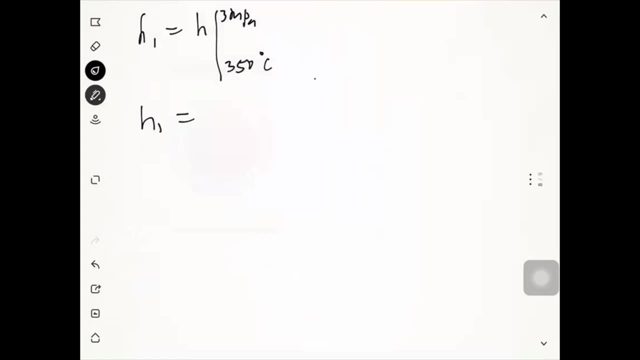 So At point here, H3, We have 0.075 MPa, Or that is H3 at This H3, This H3 at At this particular pressure. So H3 is H3 at 4 Per kilogram And our V3 Is The Vf. 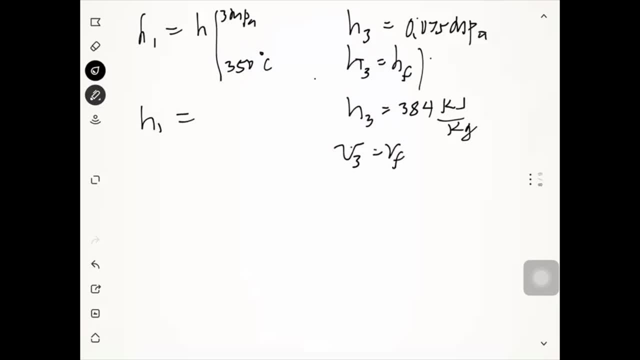 Which is 0.001037. This is in kilojoule. Oh no, that is in. This is in meter cube Per kilogram. Okay, So On the same table, Each one will be 3115 kilojoule Per kilogram Per kilogram. 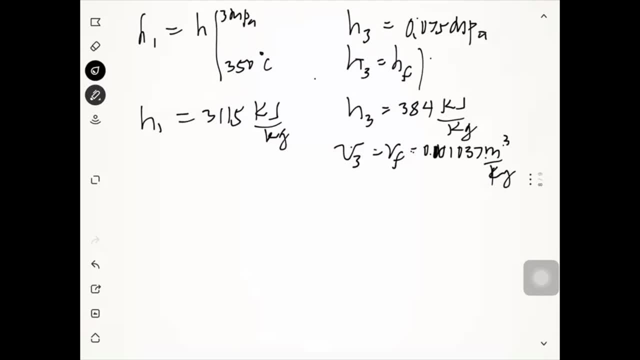 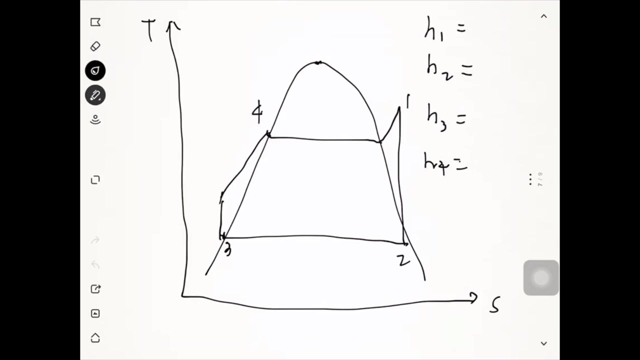 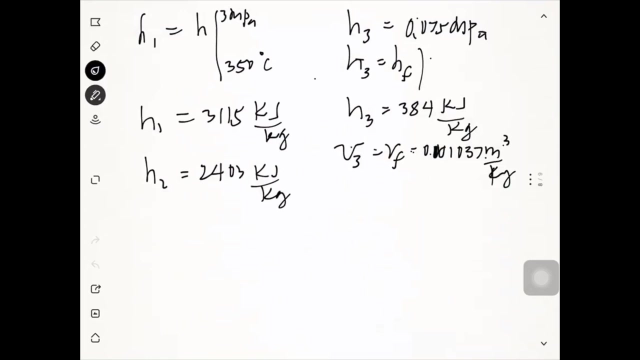 And, and we have our H2- our H2 would be 2403 kilojoule per kilogram. so we have H1 and we have H2. so you can also calculate the H4. how are we going to calculate H4 here? okay, there's no need to calculate the H4 because 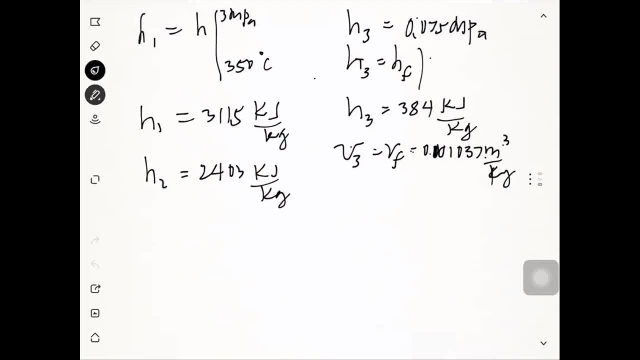 we have the work net. now it's work of the turbine minus work of the pump. okay, work of the turbine would be H1 minus H2 minus work of the pump. work of the pump would be point zero, zero, one zero, three, seven times the pressure, four minus pressure. 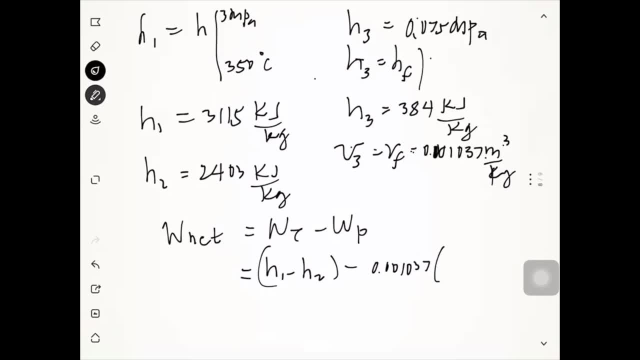 three for pressure. four is three megapascal and that is three thousand minus 75. we have our work net. since this is a very small, that can be in English. so you have the work, or this is three, okay here. so the work net would be this. 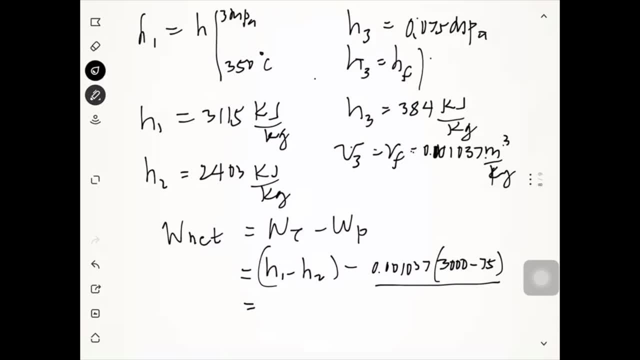 one, three, one one five minus h2. h2 is two four zero, three minus this, one minus three. so this is seven zero nine kilojoules per kilogram. that is the work net of our Rankine cycle. okay, so we're going to solve also in the Q in. 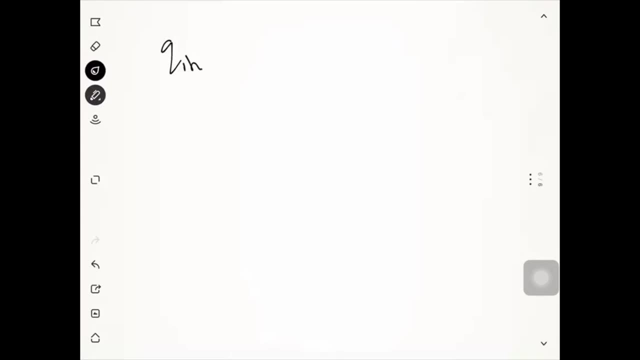 our Q in would be h1 minus h3. our h1 is given. we have okay, okay, okay, or each one, we, or each one. we have our Q in. we have h1 minus h3. okay, this is minus. that is to work with the pump, okay. 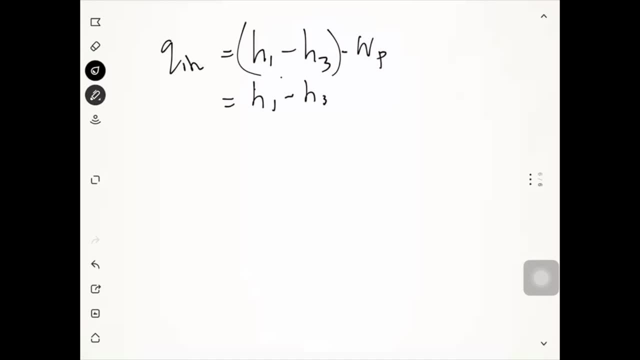 so that is three, one, one, five minus three, eight, four point three, ah, three, four, that is minus point three minus three. so we have our Q in that is two, seven to eight. so we have our Q in that is two, seven to eight. we have our Q in that is two, seven to eight. 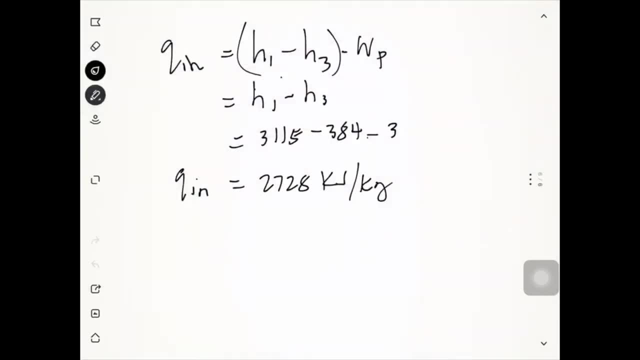 you have to buy the work net and we have the value of our Q in for kilogram. so we can solve now the thermal efficiency over Rankine cycle, that is work net over Q in, and this is two, seven to eight killings per kilogram and this is 709 over 2728. 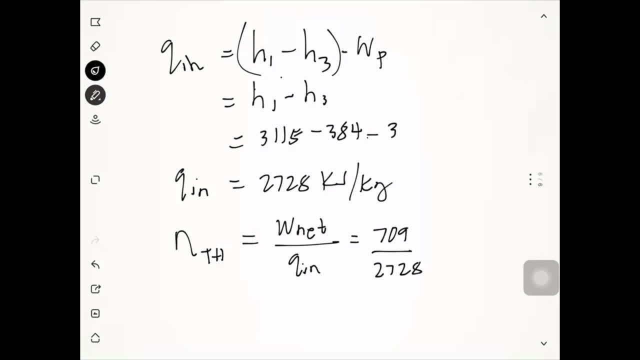 okay, so that would be 0.2599, or that is 25.99 percent. so so we have the answer for our rank and cycle: 25.99 percent. um, as we're going to draw again, the t is diagram for our rank and cycle. 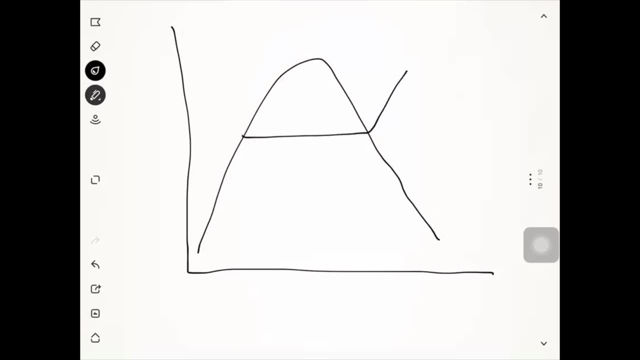 okay, so that one we have this: 0.1, 0.2, 0.3 and 0.4. so, uh, we know that this is an ideal cycle for vapor, power cycles, gear and pencil. and you know for a fact from our knowledge of the second law of thermodynamics, because of its irreversibilities, for example. 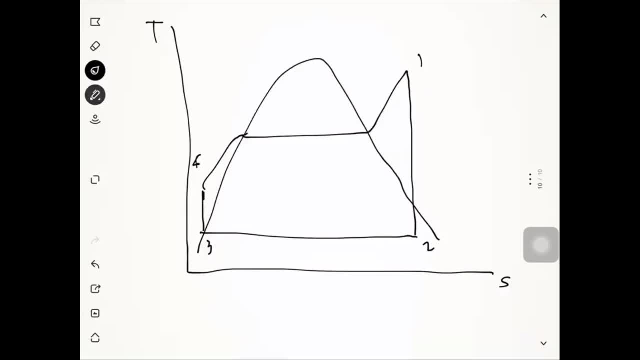 the fluid friction causes pressure drops in the boiler into condenser. and so we can see: the fluid friction causes pressure drops in the boiler into condenser and in the piping in between and for the various components, the heat loss from the steam to the surroundings as the steam flows through the various components and the division of 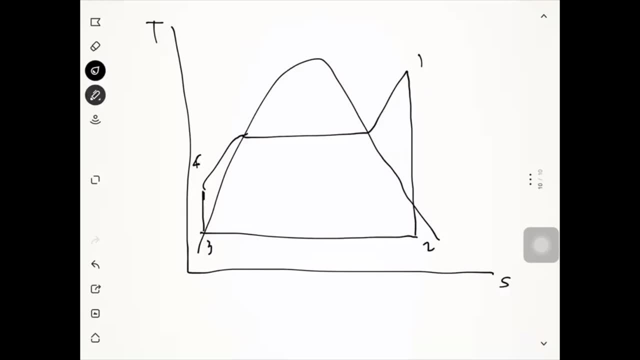 actual pumps and turbines from the isentropic plants can be accounted for by utilizing isentropic efficiencies. So if we have the isentropic efficiencies, this would be like this one, this dotted line, and this one, And this would be my 2 prime and this would be my 4 prime. that is, the actual before power. 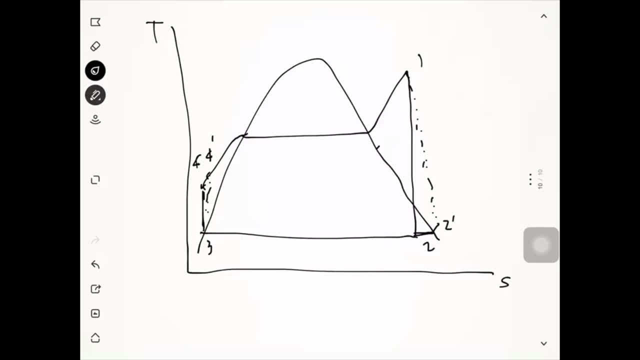 cycle. Okay, So also, as we mentioned earlier here, due to the losses, that one, this would be our 1 prime, And also this one, it would be the. this would be the division for the actual versus the ideal cycle. 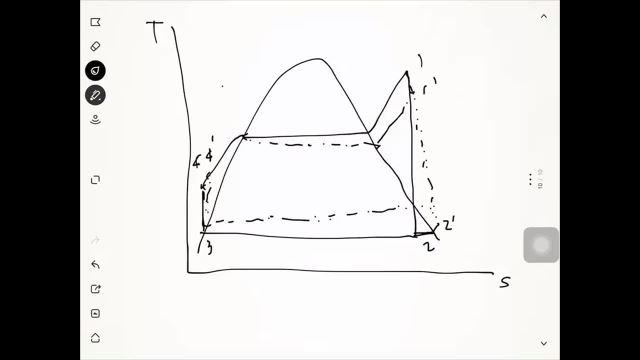 So, but of course we assume for our analysis, we assume that this is the ideal cycle. Okay, So this is the ideal cycle. Okay, This is the term of, but because it has no significant effect, that for the isentropic efficiencies this would be the should be our diagram here, this dotted. 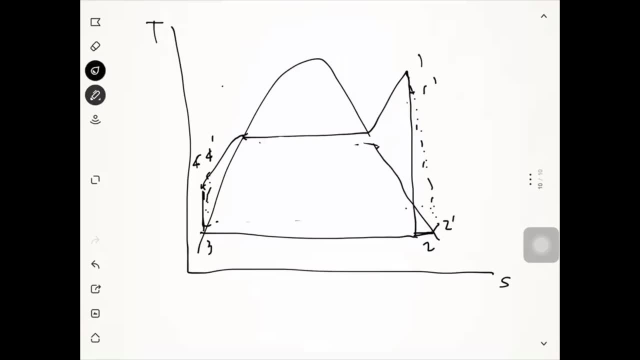 line. Okay, For example, we have given efficiencies for a pump and we have given a centrifugal efficiency for a turbine. okay, so now that is the division for the division for the power cycle, actual versus the ideal cycle. okay, so question: since runtime cycle is the ideal? 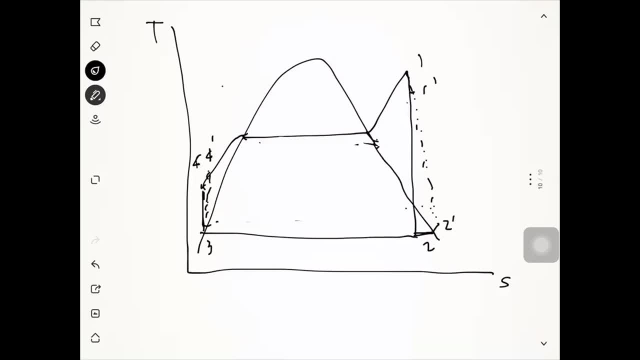 and we have some ways to improve its efficiency. okay, so what are these ways? this number one is here: by increasing, by lowering the condenser pressure. so we lower the condenser pressure. okay. so when we lower the condenser pressure, this will be a work. so when we lower the condenser pressure, this would be a work. 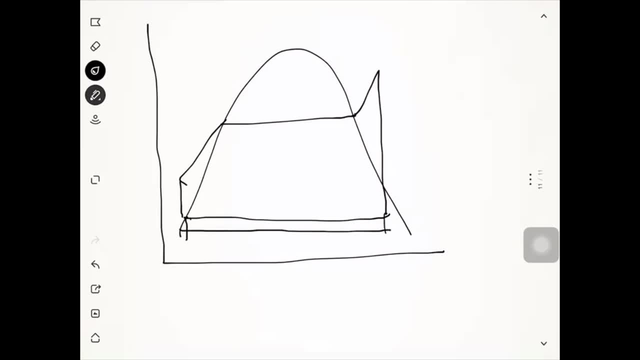 one point, one point two. so 2 prime, this is our 3, this is our 3 prime and this would be our 4 prime. this is our 4 and this is our. ok, this is our 4 prime here. 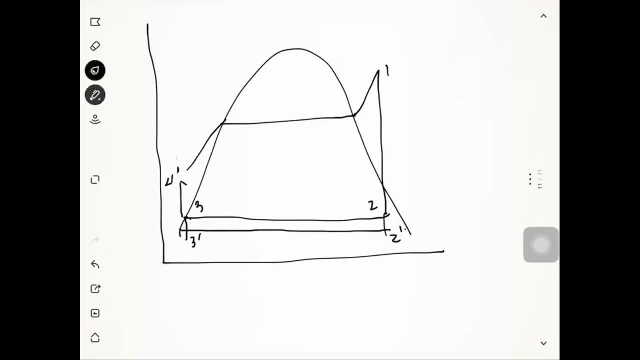 Our 4 and this would be our 4 prime. So by by, this would be this area. this would be the increase in our work net where we lower the condenser pressure. ok, So then we at the diagram, since our thermal efficiency would be the walk net over the Q, added over the Qn. so 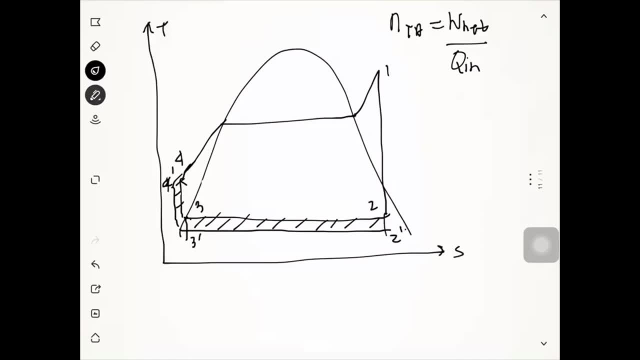 since the thermal efficiency would be proportional to our walk net. so since there is an increase in the walk net, so our thermal efficiency efficiency would be. we would also increase. okay, so to illustrate that one, we will continue by: for example, we would lower the pressure from 75. 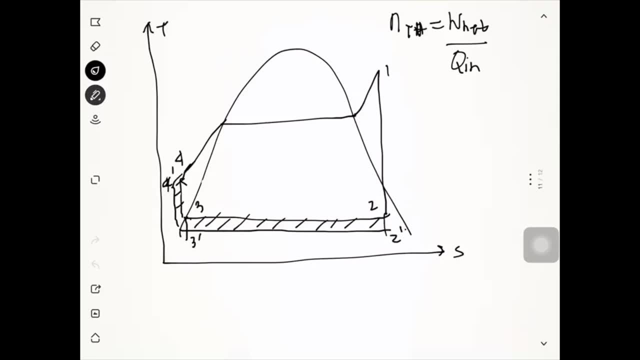 kilopascal down to 10 kilopascal say. let's say 10 kilopascal so we will solve. therefore, trying to show if it really, If the efficiency would increase. okay, this is, this is our 75 kilopascal condenser power. condenser power. 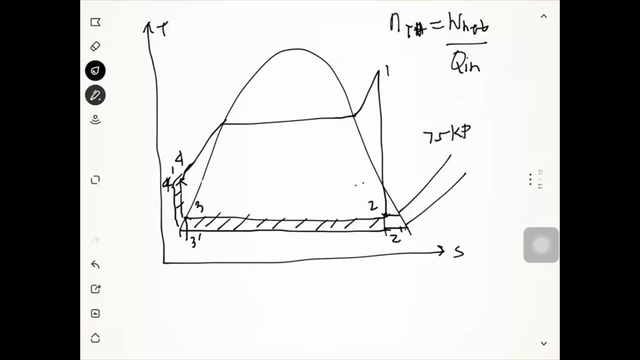 pressure and this would be the hour: 10 kilopascal. so we lower that one, okay. so based on this thin table, again we have the H here, the H2 prime. H2 prime would be 2136 kilojoules kilogram based on this thin table. so now 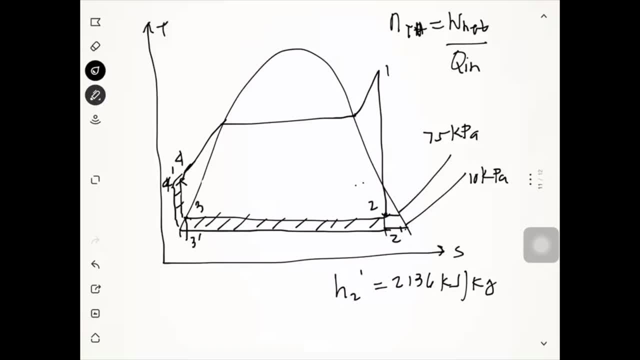 we'll compute its efficiency, which is true. that efficiency would increase. you have the work net. you have the work net. that is 3115 minus 2136 minus 3 and that is 2136 976. this is in kilojoules per kilogram. 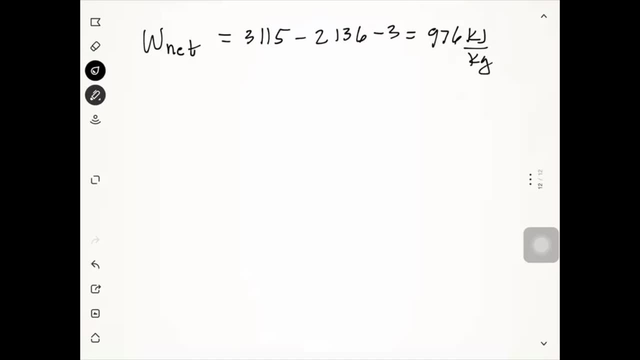 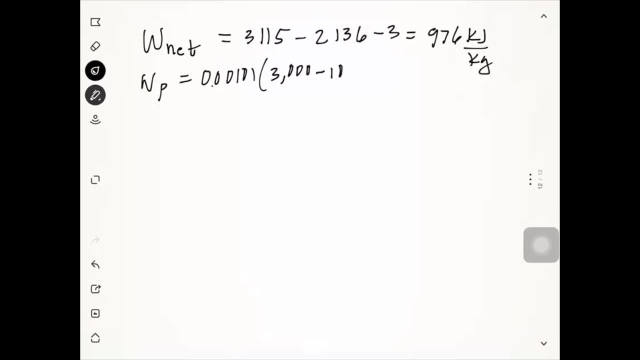 times the three nico pascal, this 3000 kilopascal minus ten, okay, and this is also three, and we have our Q in is 3154 and we have our Q n is 3215: 3154 minus 192, minus 3, okay, so that is 2920 kilojoule per kilogram. 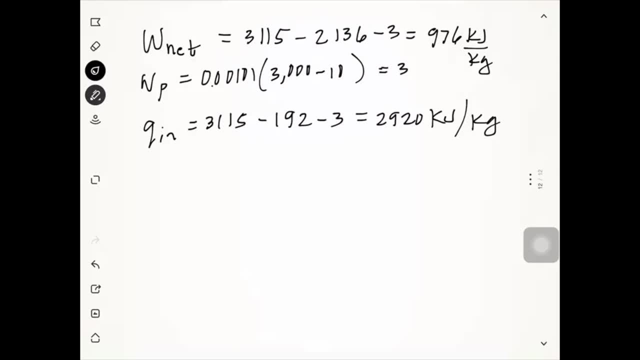 Okay, so we can compute the efficiency now. The efficiency would be 976 divided by 2920 times 100 percent, So this is 33.42.. So it is true this in our previous example, so our efficiency is. 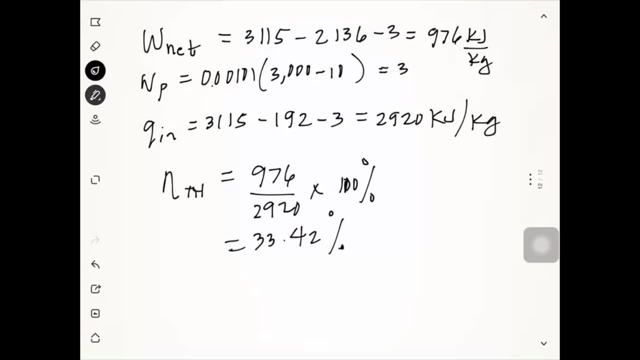 Actually it is just zero. have the 25.99%, So it would increase. there is an increase from 25 to 33.42.. So we can say, therefore, that the effect of lowering the condenser pressure would also increase. 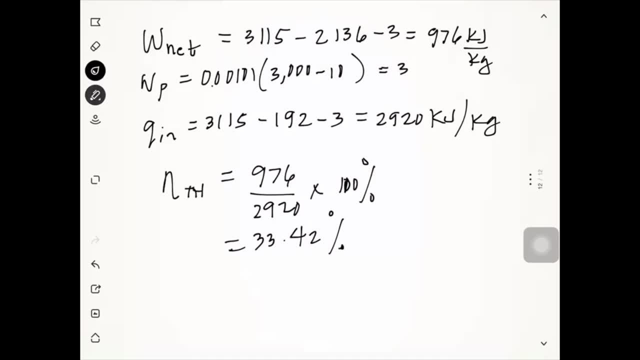 the thermal efficiency. So, but there is a limit when lowering the pressure for the condenser. that is its limit. its limit would be a, the lower limit for the condenser pressure that can be used. can it be lower than the saturation pressure corresponding to the temperature of the cooling medium? So you would, for example, 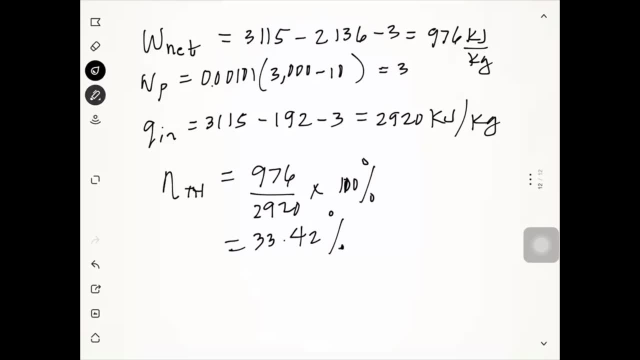 you consider a condenser, a condenser, a condenser that is to be cooled by an early river at 15 degrees Celsius, allowing a temperature difference of 10 degrees Celsius. for effective heat transfer- that's common- The steam temperature in the condenser must be above 25 degrees Celsius. Thus we have, we have 3.2 kilopascal. 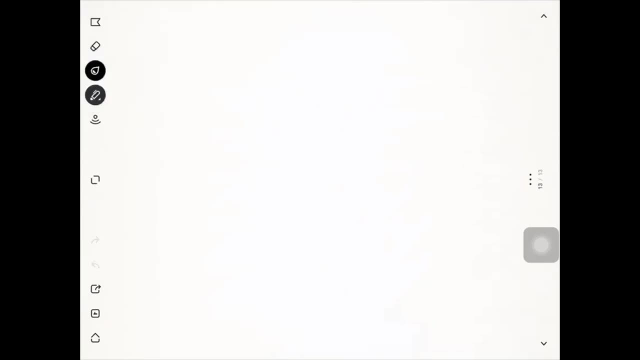 So we have 3.2 kilopascal. So we have 3.2 kilopascal And if we have hot hot ripple associated with it, we would have the lower limit of 3구나 Celsius. OK, This is not no. 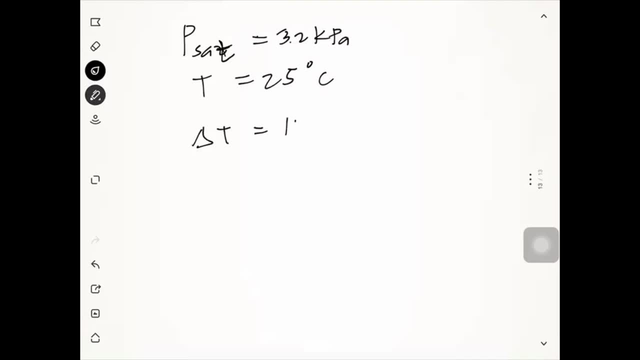 In fact, the need of this pressure will be lower than 3.2 kilopascal. This is because the voltage of condenser is much lower. 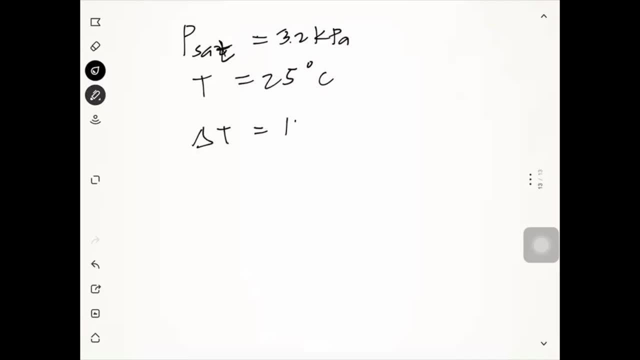 degrees Celsius. so again, the difference in the delta T here for effective heat transfer, that this would be 10 degrees Celsius. so if you're the temperature of your river for your condenser is 15, then for example you have 25. so this delta T is our assumption for effective heat transfer. this temperature and pressure would vary. depends on the source, the source of the term water entering our condenser. you have to maintain the 10 degrees delta T, okay, so the effect of lower than this, the saturation temperature or the saturation pressure would be leaking. there's, there's leakage, leakage of the. this would it would be air leakage for the condenser and that air leakage. 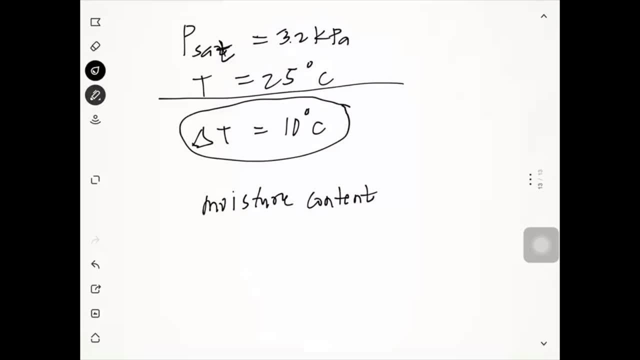 would contribute to increase on the most, increase on the moisture content. moisture content and, as we discussed, the increase in moisture content can cause erosions in our turbine blades. okay, so so another. there's another thing? so so another. there's another thing, so so, so another. there's another thing, so so. 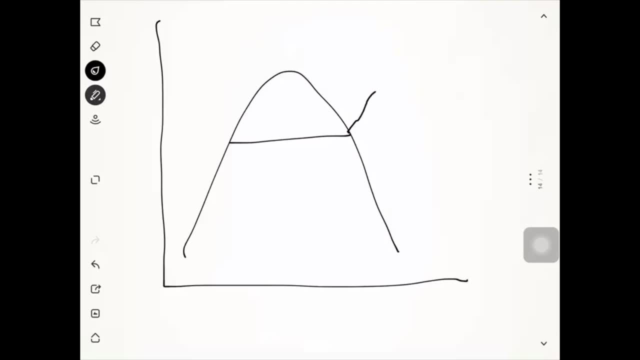 so, so, so we would, we would. we would superheat the steam to high temperatures, superheat the steam to high temperatures, superheat the steam to high temperatures. okay, so what would be the effect? so, what would be the effect? so what would be the effect when we superheat? 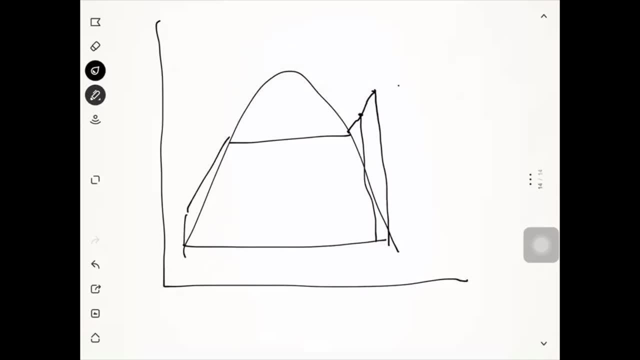 when we superheat, when we superheat the steam, the steam, when you separated one from this point: 0.1, 0.2, 0.3, 0.4. this is our 1 prime. this is our 2 prime. 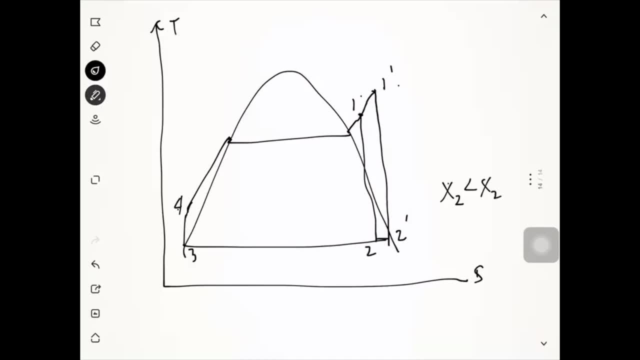 as you can see in our TES diagram here, if there is superheating in our steam entering the turbine so as it expands, this will contribute in increasing our quality, since our quality x2 is lesser than the quality x2 prime or x2 prime is greater than x2. 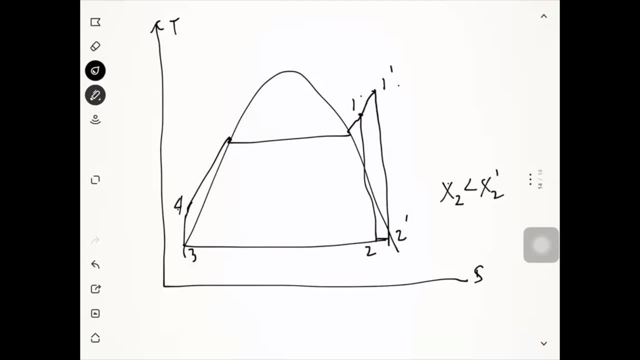 ok, so again we will illustrate that with an example. for example, we will assume a temperature for x2 1 prime. for example, we have, we have here 600, we have 600. here we have a temperature of 600. so from our gibbon for our previous problem, 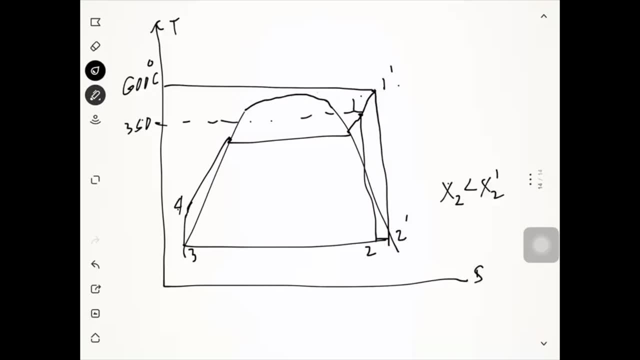 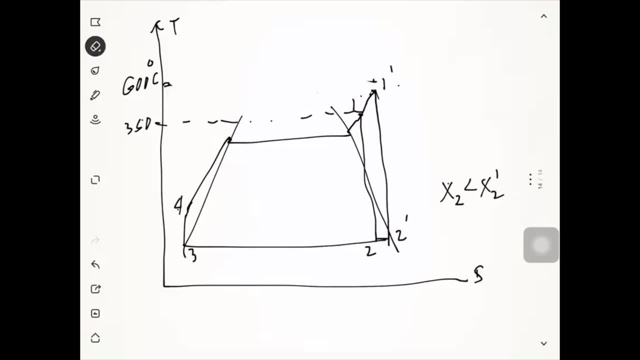 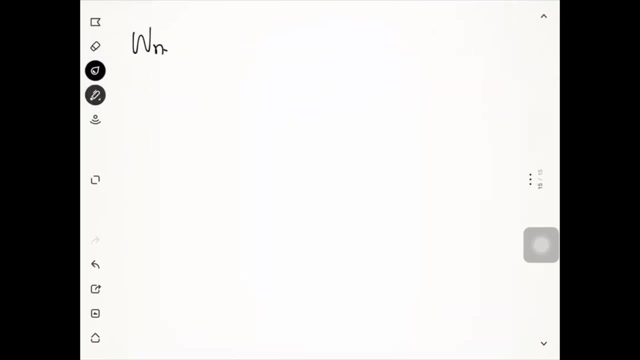 and 3 negapascal that is in our steam table. when we look at our steam table that is 3683 kilojoule per kilogram. Okay, So we compute again the work net. Our work net would be is 3683 minus 2380 minus 3 in the work over pump and that is. 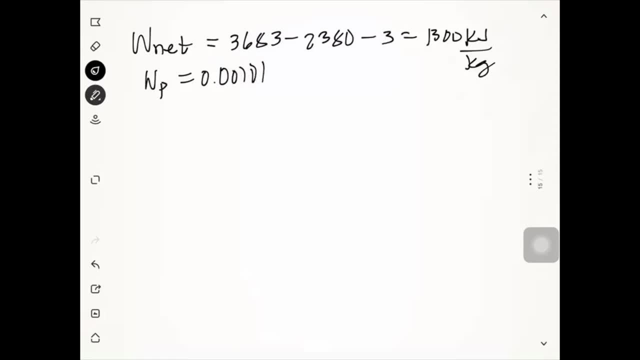 1300.. Okay, So we compute again the work net. Okay, So we compute again the work net. Okay, So we compute again the work net. So we compute again the work net. kilojoule per kilogram. 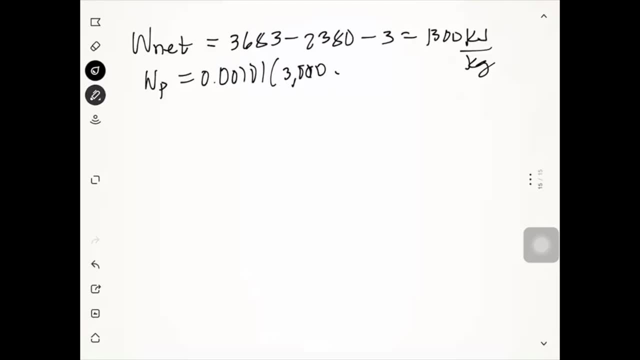 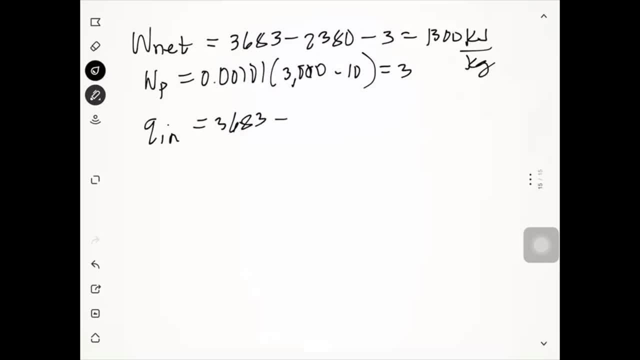 0.00101.. times the 3,000 minus 10, this is 3, and our Q would be. Qn would be 3683 minus 192. minus 3, this would be 3488 kilojoules per kilogram. so 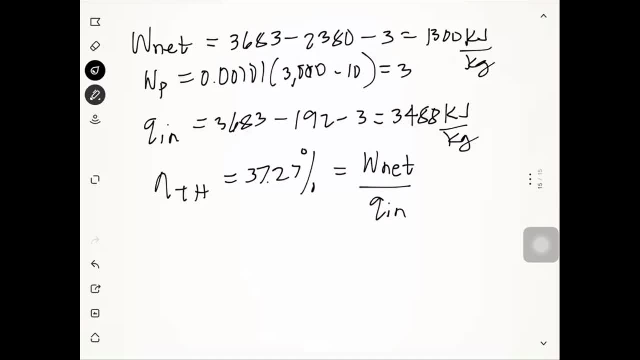 our efficiency would be 37 point 27 percent. this is rock net over Qn. okay, so we have shown that by increasing the boiler or the the, by increasing the boiler temperature or separating the steam inlet to the turbine, hence we have the increase of thermal efficiency. 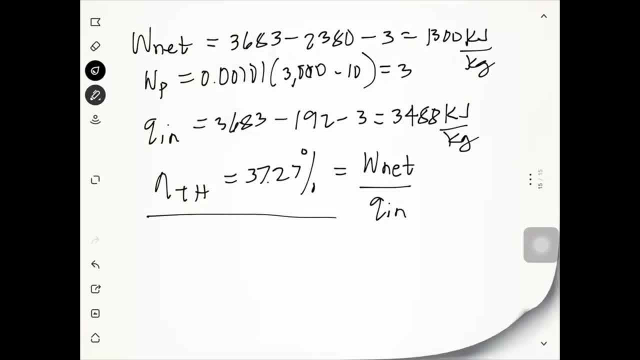 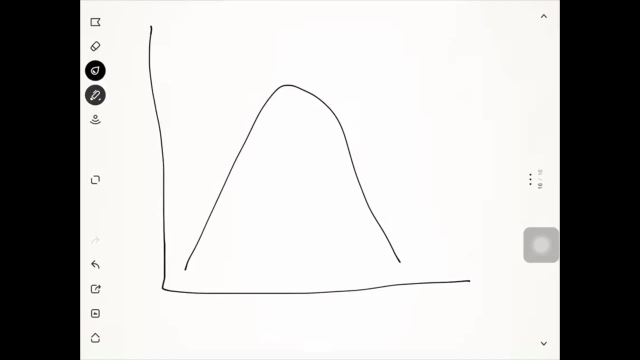 now we have, last, our last condition: by increasing the, by increasing the boiler pressure. you have to increase the boiler pressure. So by increasing the boiler pressure, we have to draw the TS diagram, that one, so increasing the boiler pressure, that one At the same temperature. 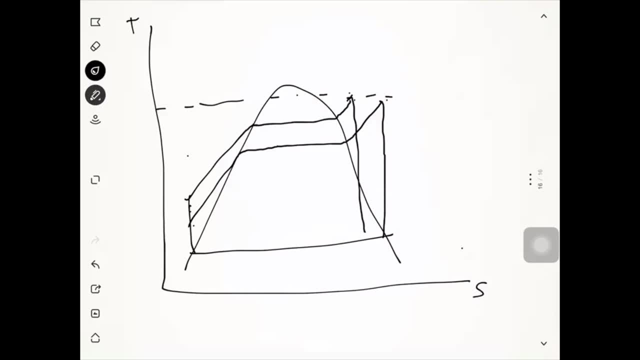 So TS diagram, So TS diagram. So TS diagram To increase the boiler pressure here at 15 MPa. this one, This is our 3 MPa. Ok, So by our steam tables, this is our 1 prime, 1,, 2, 2 prime, 3,, 4,, 5,, 6,, 7,, 8,, 9,, 10,, 11,. 12,, 13,, 14,, 15,, 16,, 17,, 18,, 19,, 20,, 21,, 22,, 23,, 24,, 25,, 26,, 27,, 28,, 29,, 30,, 31,, 32,, 33,, 34,. 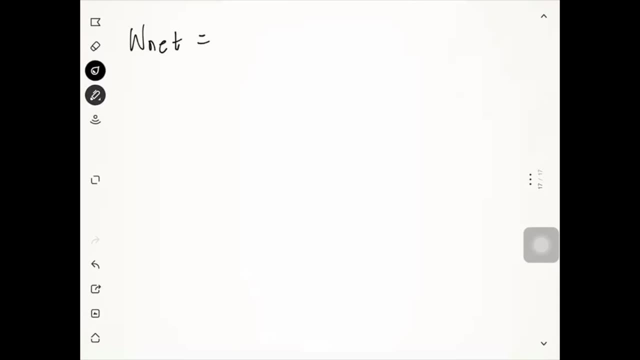 3583, kilojoule per kilogram. Okay, you have. you increase the boiler pressure from 3 to 15 micropascal, So we will compute now the work net: 3583 minus 2115 minus 15.. 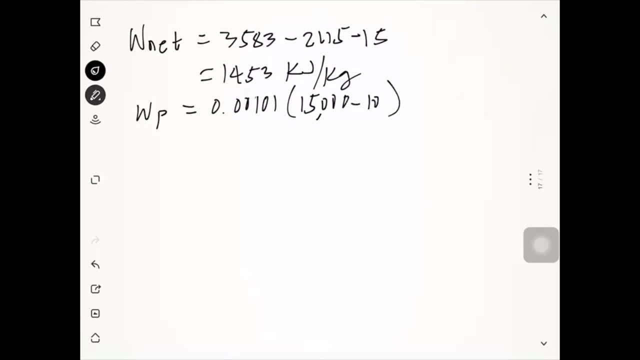 This is 1453 kilojoule per kilogram Workable pump. that would be 0.001.. 0.00101.. 15.. 1,000 minus 10.. So this is 15.. Okay, and our Q in would be 3583 minus 192.. 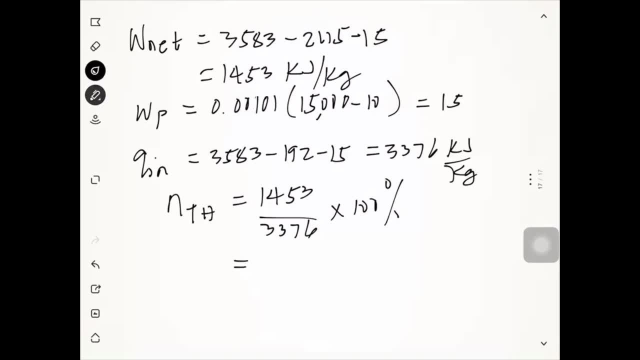 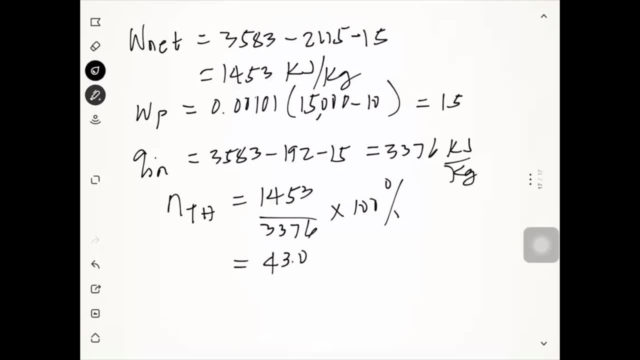 This is 3,, 3,, 7,, 6.. Kilojoule per kilogram And our efficiency would be 1,, 4,, 5,, 3.. Over 3,, 3,, 7,, 6.. 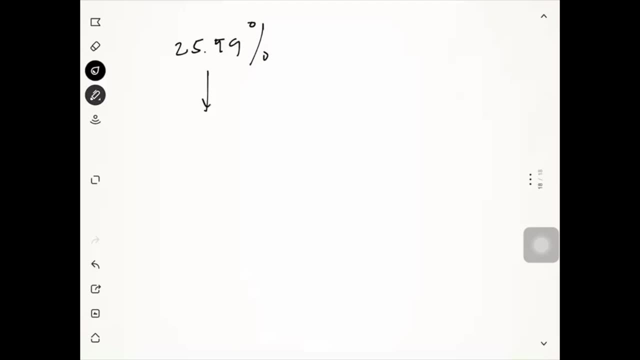 3, 3,, 7, 6.. this would be 43.04 kilojoules per kilogram. okay, so you know that we have three cases, and from 25.99% it's going to increase to if you lower the condenser pressure.